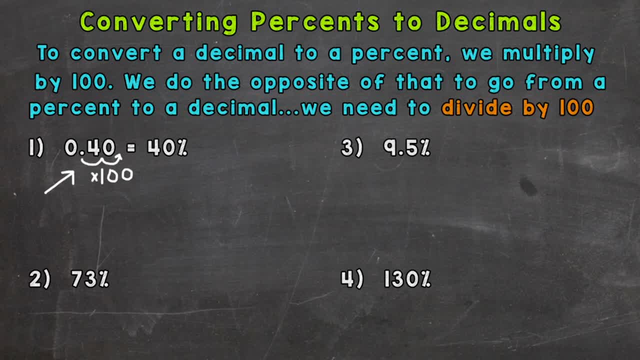 multiplying by 100. We do the opposite of that, to go from a percent back to a decimal. So we need to divide by 100. So, for example, number one: here again, we started with 40 hundredths. We multiplied by 100 to get 40 percent. So we need to move the decimal back two times to the left, which is: 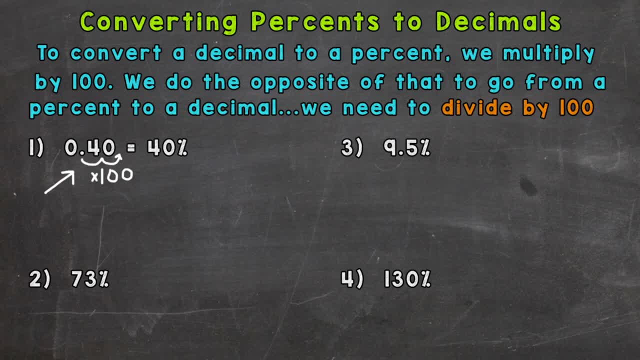 dividing by 100 to go back to a decimal. So we do the opposite of that, to go from a percent to a to a decimal, so one, two and we would go back to the equivalent decimal to that percent. so all you need to do is divide by a hundred to go from percent to. 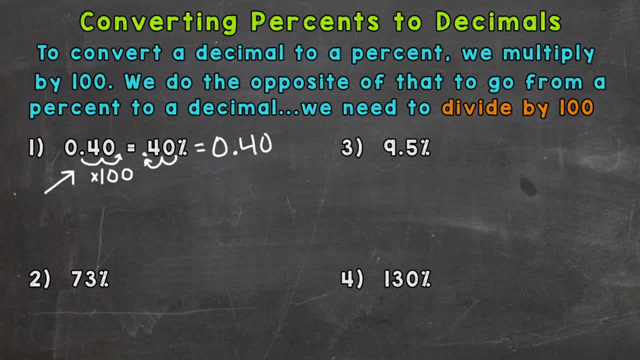 decimal. so number two: we have 73%, so we would need to move the decimal twice to the left, which is the same as dividing by 100, 1, 2, so our decimal would be 73 hundredths. for number three, we have nine and five tenths percent or nine, and 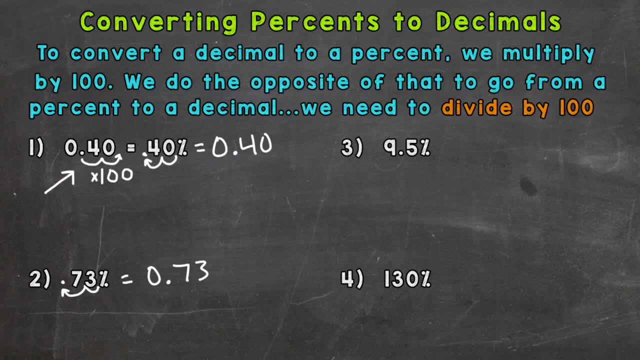 a half percent. so again divide by a hundred, or move the decimal twice to the left, one: 2. fill that gap with a placeholder zero and we end up with 95 thousandths. number four: we have 130 percent. so again divide by a hundred to get to a decimal move. 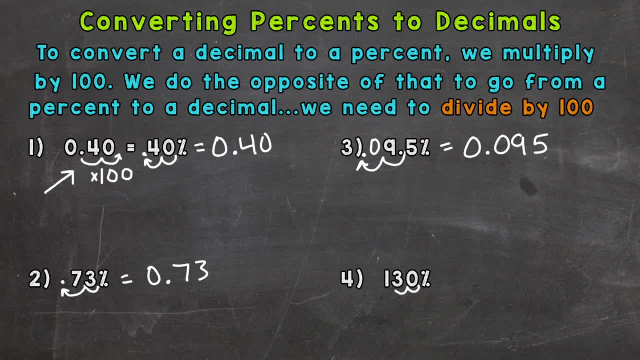 that decimal twice to the left, one, two, and the decimal is now between the one and the three. so we get one and three, thirty hundredths. so there you have it. there's how you convert a percent to a decimal, and I'll read up top again here. so, to convert a decimal to a percent, we: 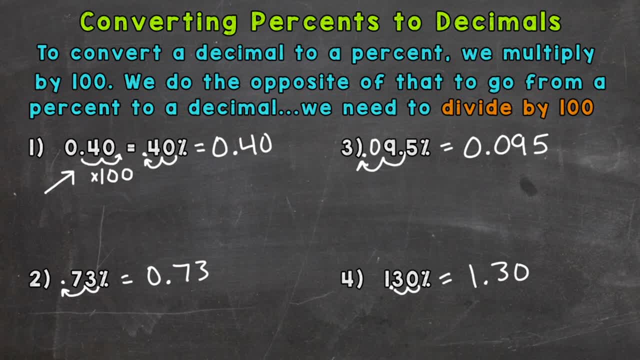 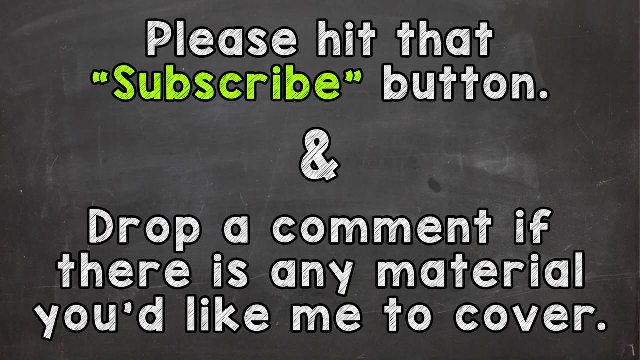 multiply by 100. we do the opposite of that to go from a percent to a decimal, so we need to divide by 100. hopefully that helped. thanks so much for watching until next time. peace you.